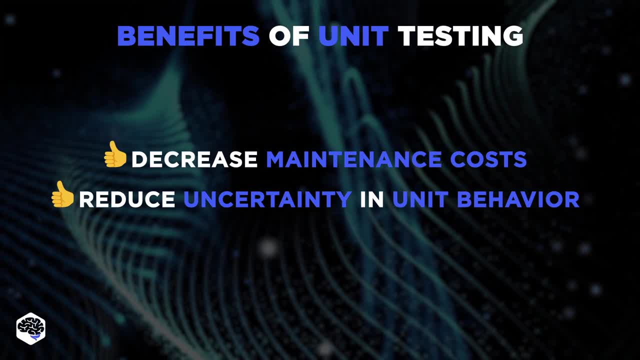 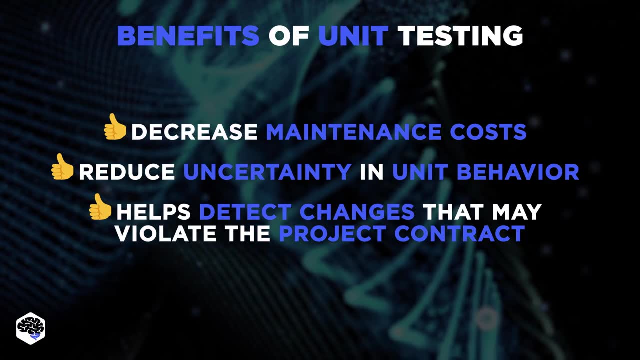 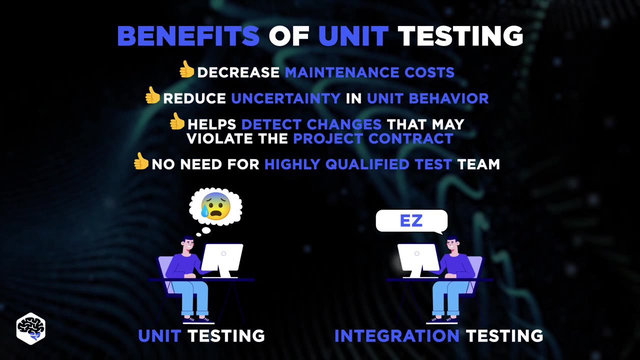 as unit testing helps to verify the performance of the underlying code. Also, unit testing helps detect changes that may violate the project contract. And finally, you don't need a highly qualified test team, As, by doing unit testing, coders don't have to manage layered interfaces or write complicated 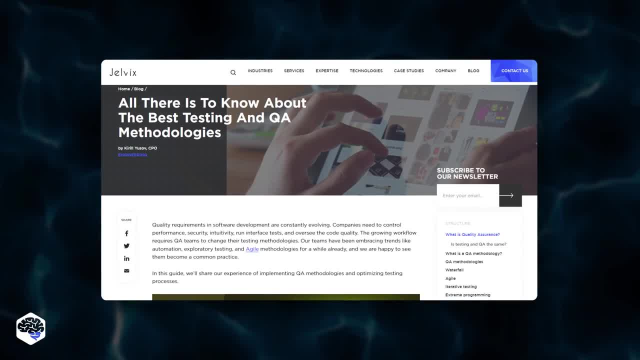 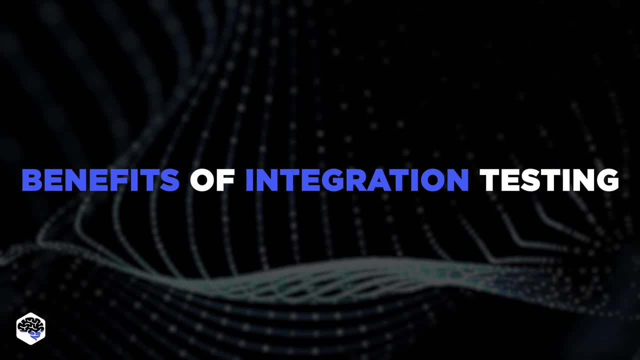 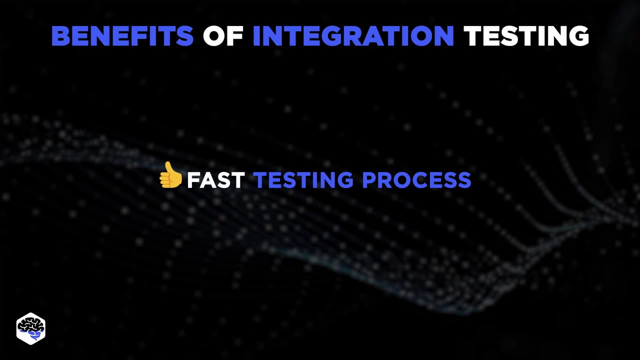 test cases. Actually, we have a great guide on the best QA methodologies and you can find the link in the description box. So what about integration testing? What are its main benefits? Well, relatively fast testing process, as this method improves speed and simplifies. 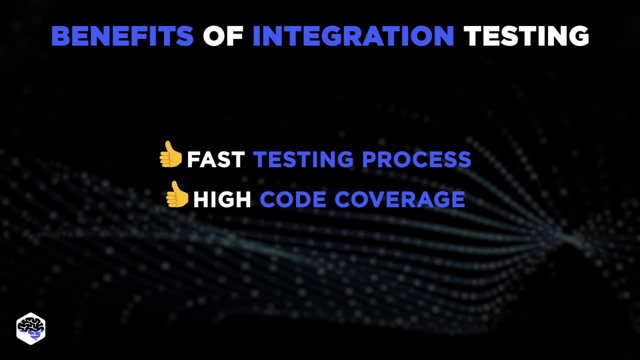 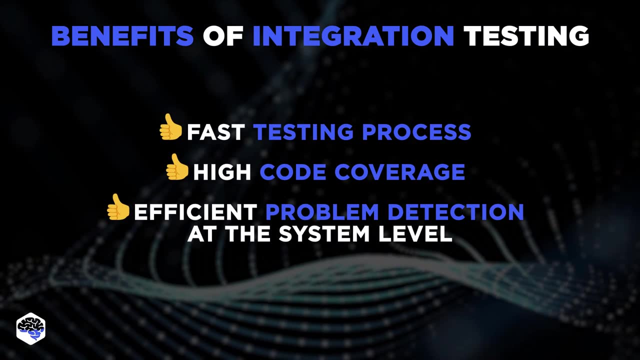 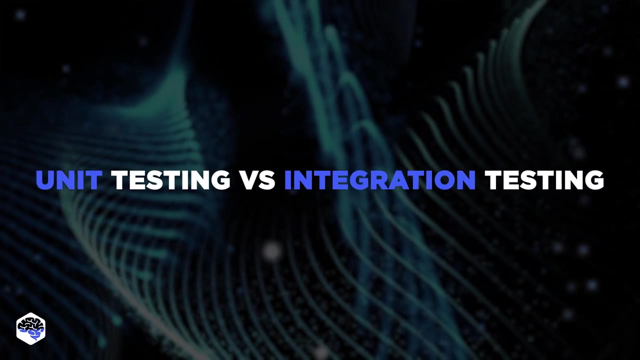 end-to-end testing. High code coverage. as integration testing has a broad scope, allowing the user to test the entire system. Efficient problem detection at the system level And detecting bugs in early development. So now let's compare unit testing and integration. 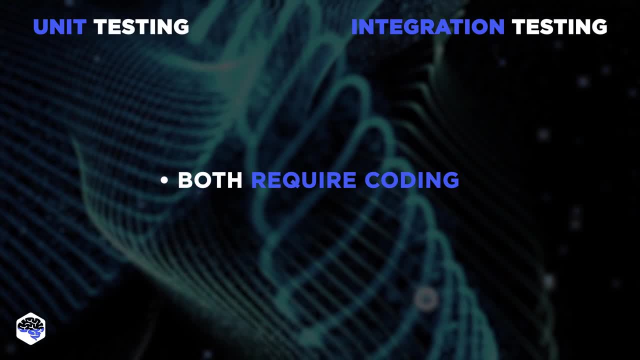 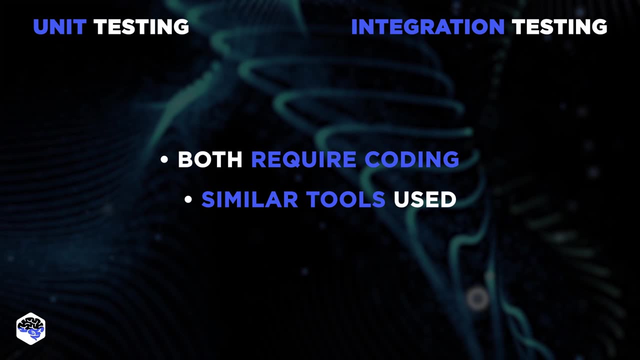 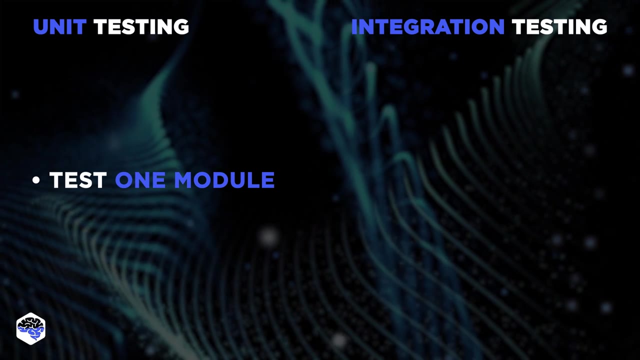 testing. These methods both require coding. in contrast to forms of testing which are based on screen recording, It's possible to perform both of them using similar or even the same instruments. So what's different about them? In unit testing, only a small module or piece of code. 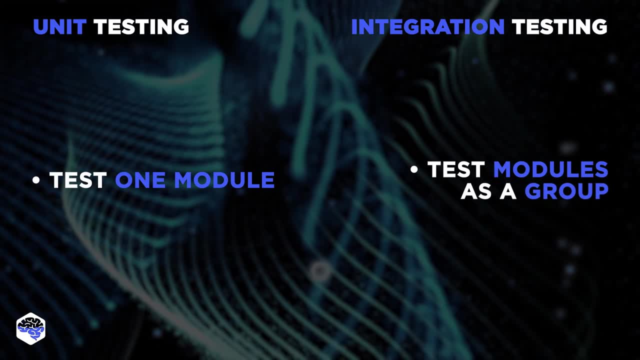 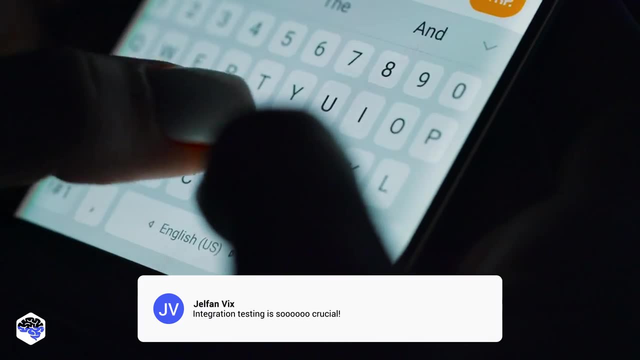 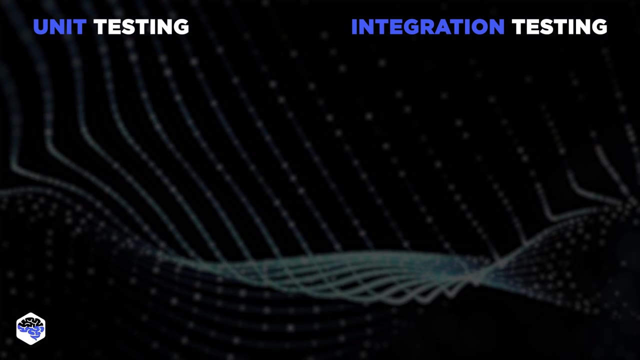 is tested. But in integration testing you test modules combined in a group. So in your opinion, which approach seems like a higher priority? one Share what you think in the comments. Unit testing is less complex than integration testing. For unit testing you'll need a single. 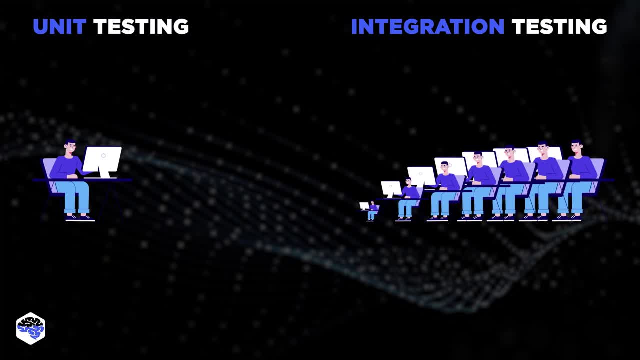 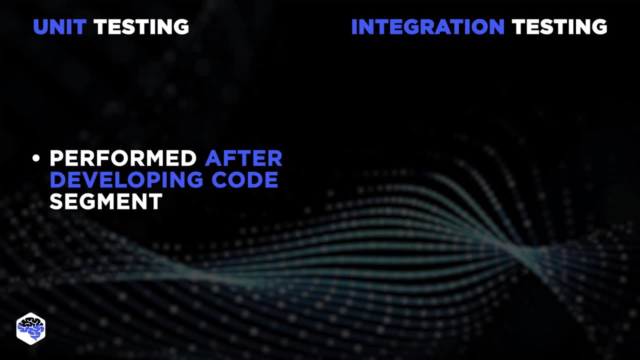 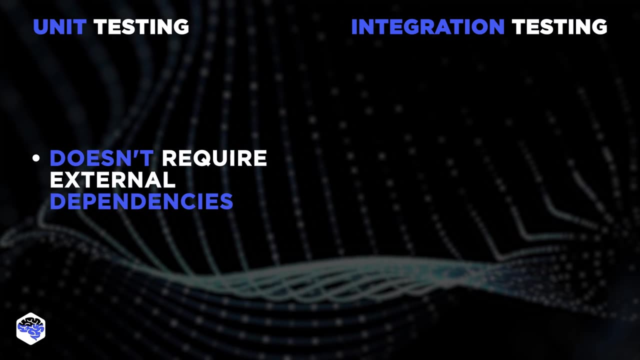 developer, But integration testing requires a team of developers. Unit testing is performed just after the development of a separate code fragment, But integration testing should be executed after unit testing and before system testing. Unit testing doesn't require the participation of external dependencies. On the contrary, integration testing requires the use 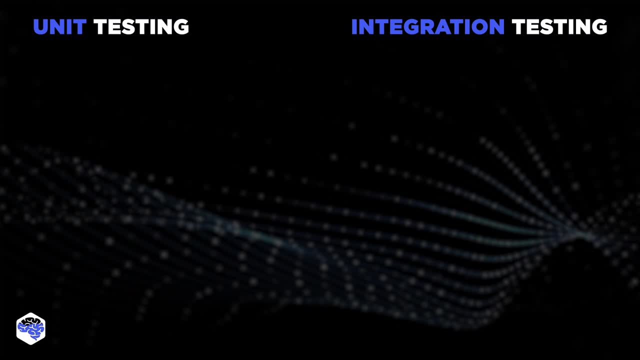 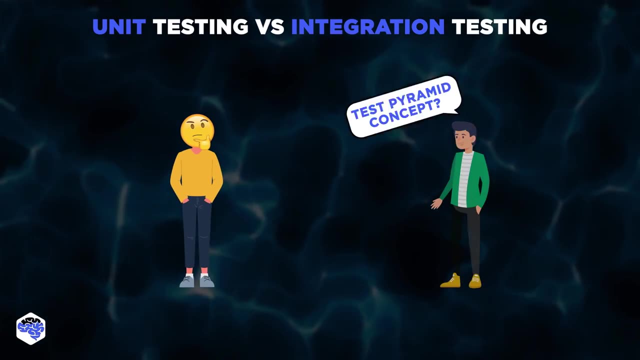 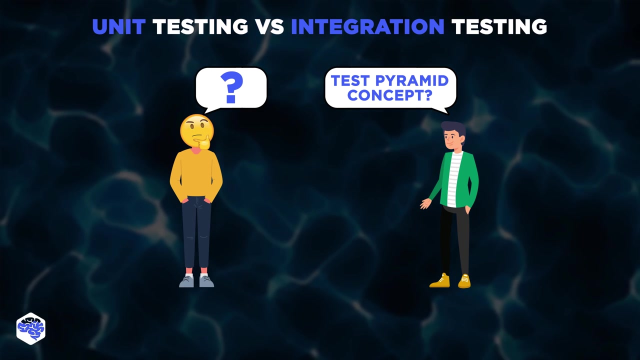 of real dependencies to perform testing. Also, unit testing is faster to write than integration testing. To get which approach suits you better, consider the test pyramid concept. that lays out the types of tests to be included in an automated test suite. It also outlines the 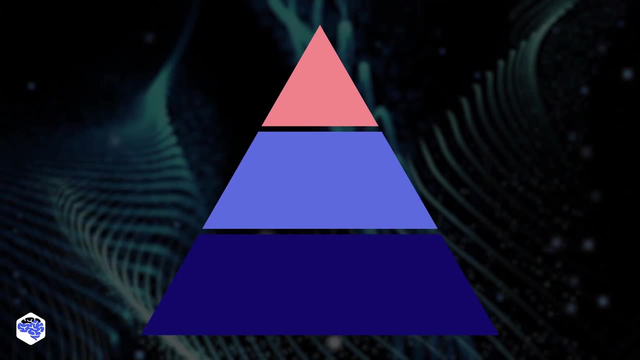 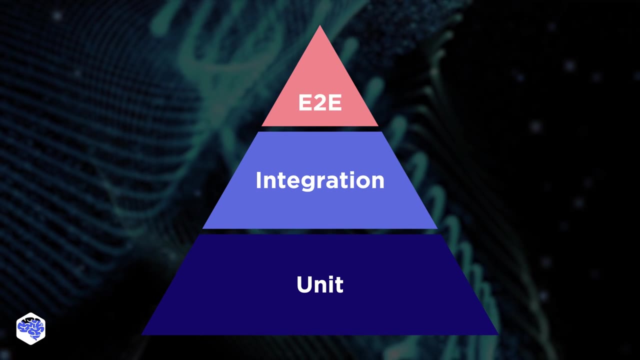 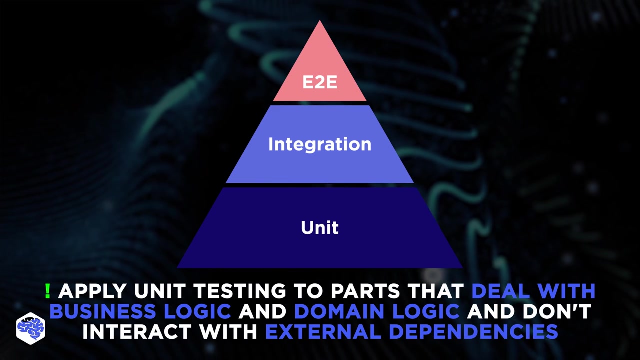 sequence and frequency of these tests. This test automation pyramid operates at three levels, namely unit tests, integration tests and end-to-end tests. Thus, maximize unit testing by applying it to the parts of your codebase that deal with business logic and domain logic.